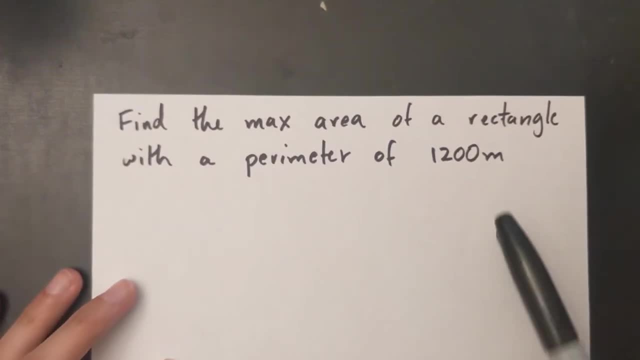 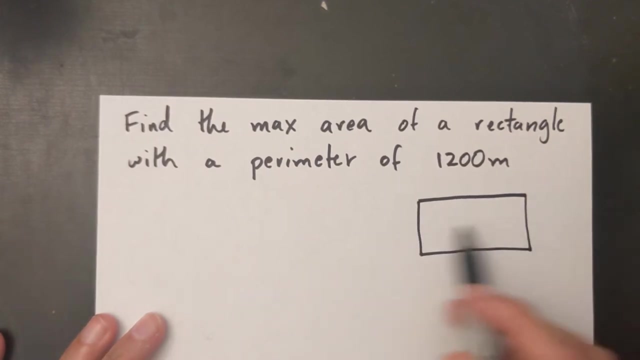 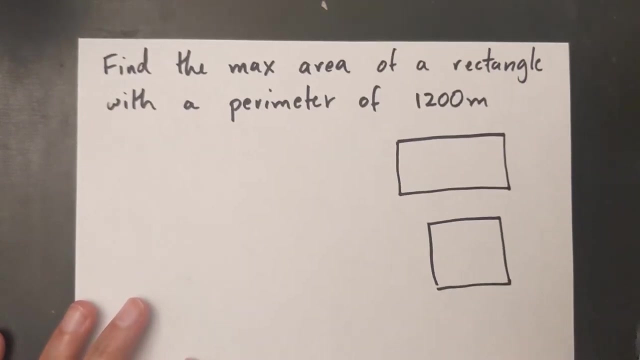 Alright. so in this problem, it asks us to find the max area of a rectangle with a perimeter of 1200 meters. So let's draw a rectangle here Now. this rectangle can be this wide, or it can be a little less wide. You don't know what the actual solution is Now technically. 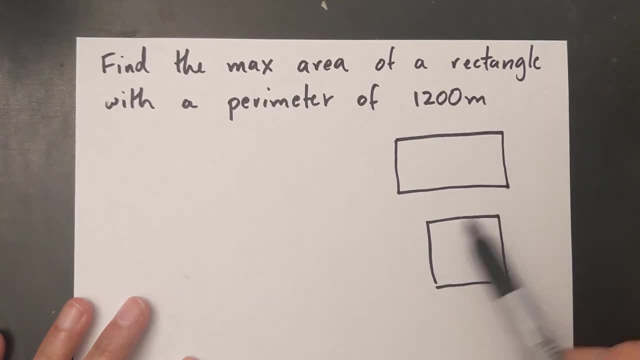 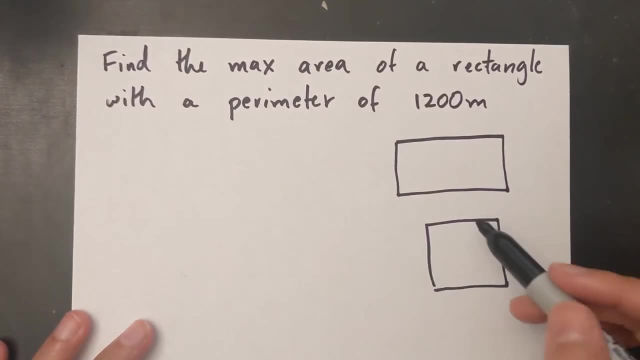 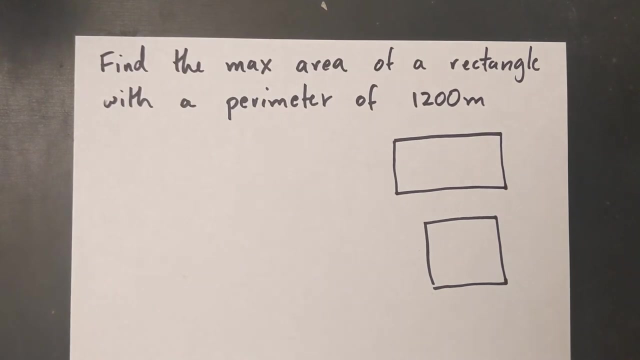 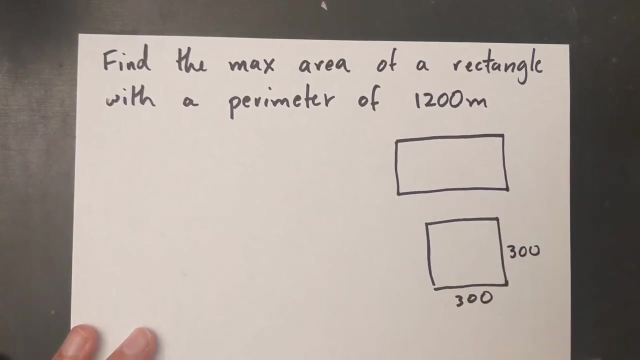 speaking without doing any calculations, the solution is always going to be a square for questions like this. So for my square, all four sides have the exact same width, So it's just 1200 divided by 4, which is basically 300.. Okay, so this is how max area can be. 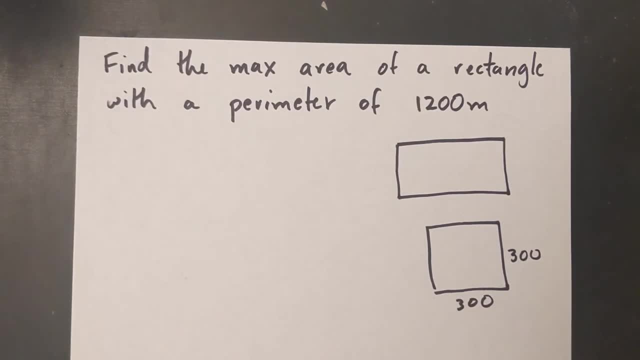 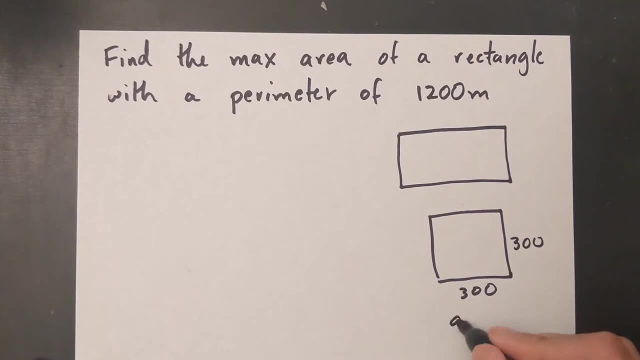 estimated or kind of. you can tell it, But we want to know how to prove this algebraically. If I wanted to find the area, I'd multiply the two 300s. So my max area would be 90,000 meters squared. But if you put this solution, 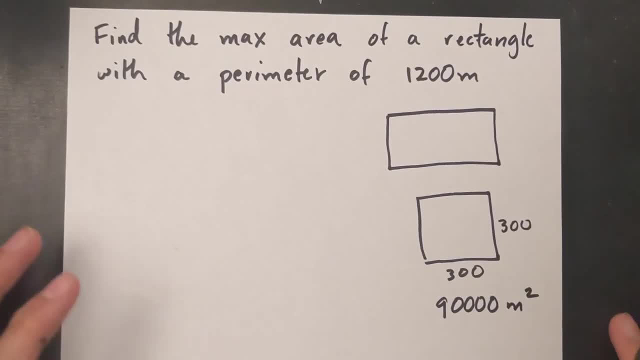 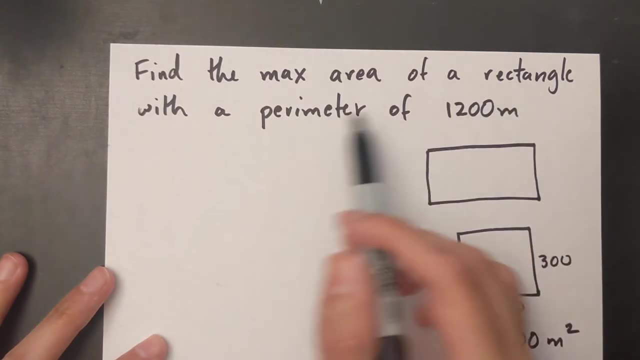 on a test, you wouldn't get any marks because you haven't proven it algebraically. So I'm going to show how to prove it algebraically in this question. The first thing I'm going to do is: I know that I have my perimeter, So I'm going to write my perimeter formula. 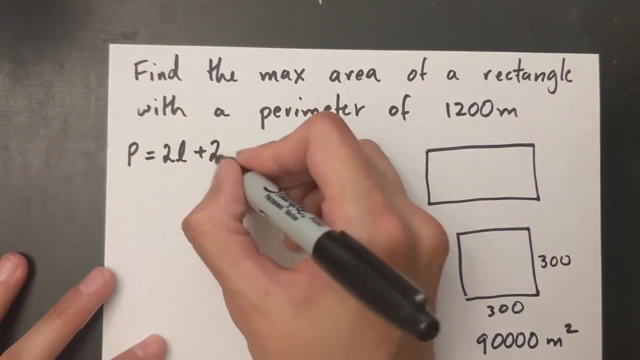 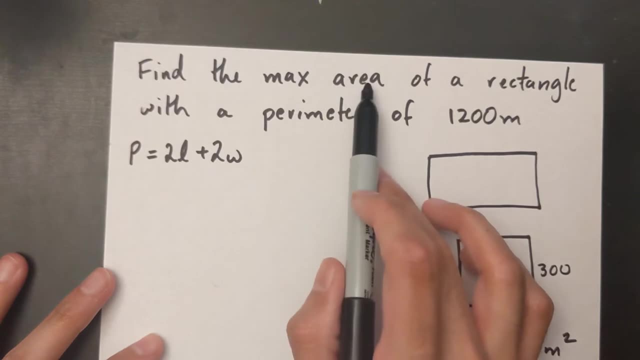 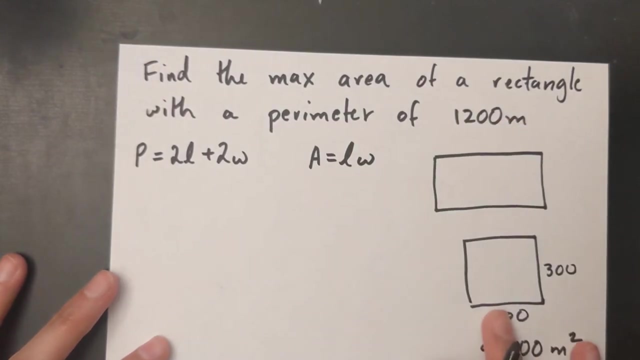 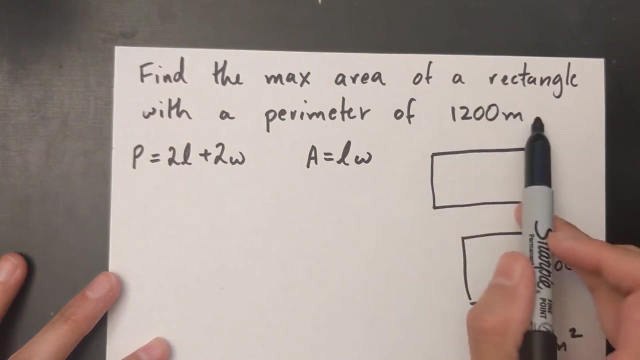 P equals P equals 2L plus 2W. The second thing I know is that I have to find the max area. I'm going to write my area equation here. Area is just length times width, And the only information I have in this question is 1200 meters squared or just meters. I'm going to replace my perimeter. 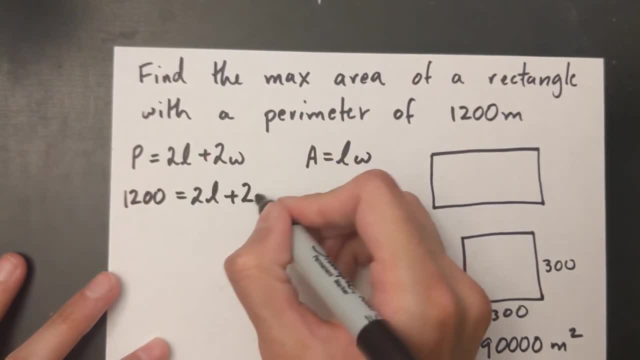 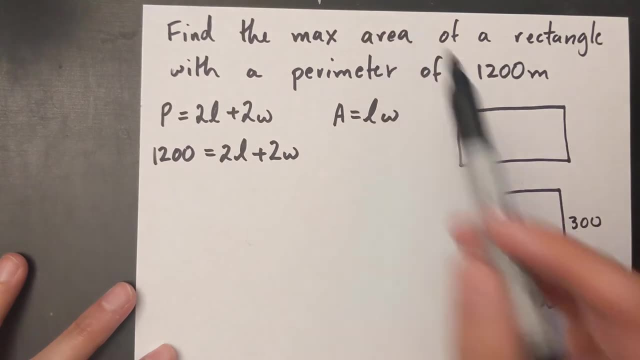 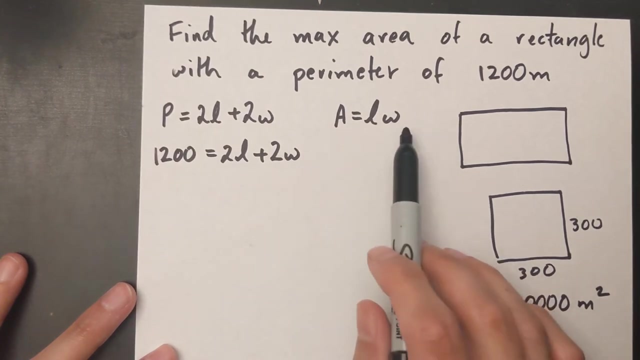 with 1200.. Okay, so this is what I've got here, And I have to use this to somehow find my max area. Well, the key to doing this is to first isolate a variable here and then sub it in this equation. 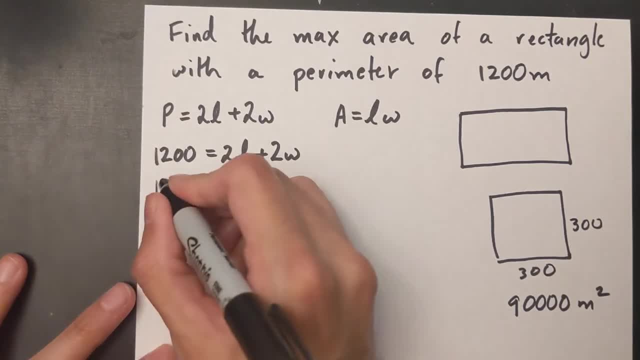 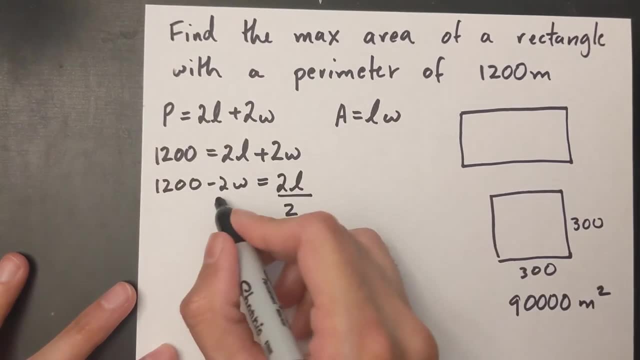 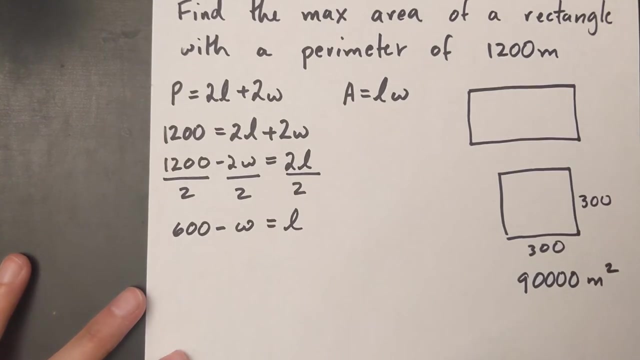 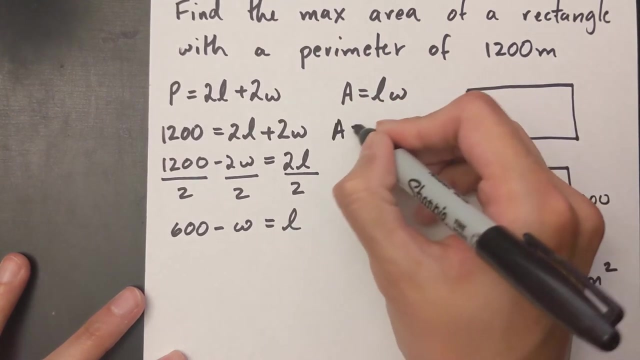 I'm going to isolate my length, I'm going to move the 2W to the other side And I'm going to divide everything by 2.. Okay, Okay, Okay, Okay. So 600 minus W is going to be my length. I'm going to substitute it over here in this equation. 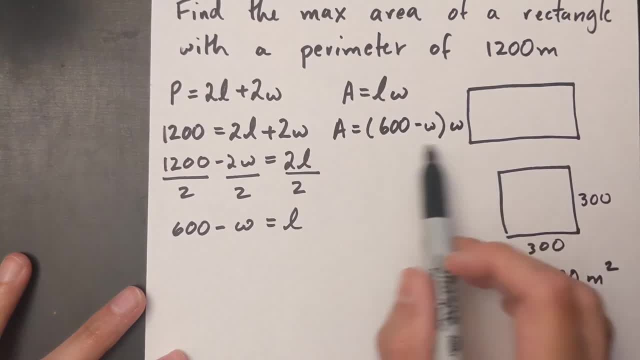 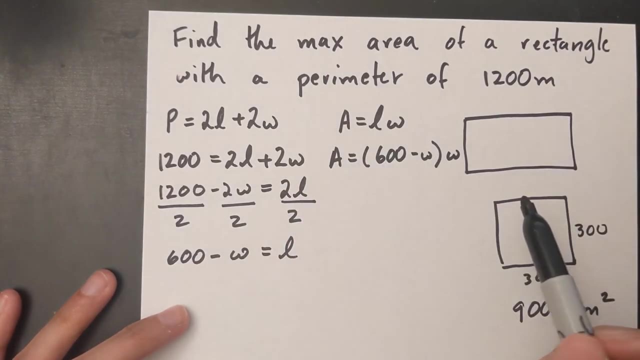 Then I'm going to expand this out or distribute it. Well, technically we don't have to. We can actually leave it in factored form. So what is this right here? This is a quadratic equation for my area and I need to find my max area. So this is already in factored form, so I can tell my solutions for. 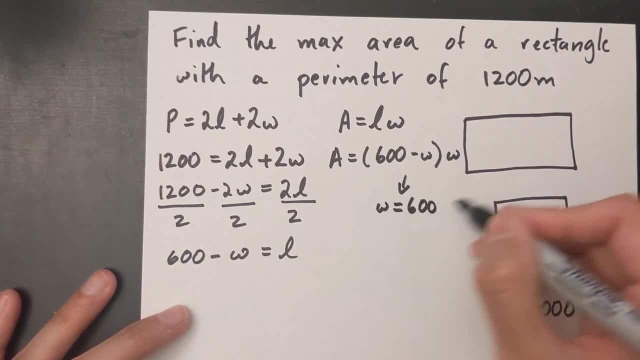 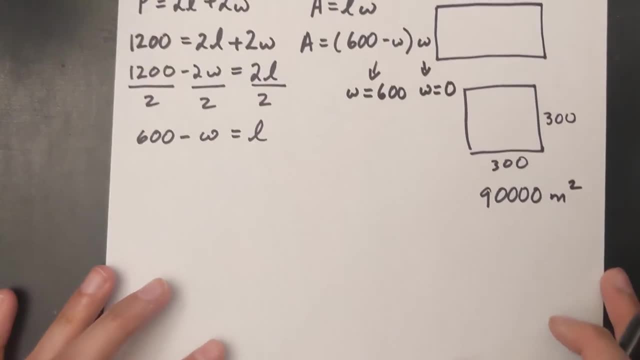 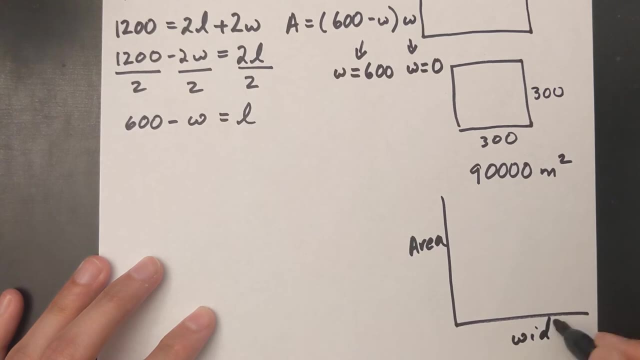 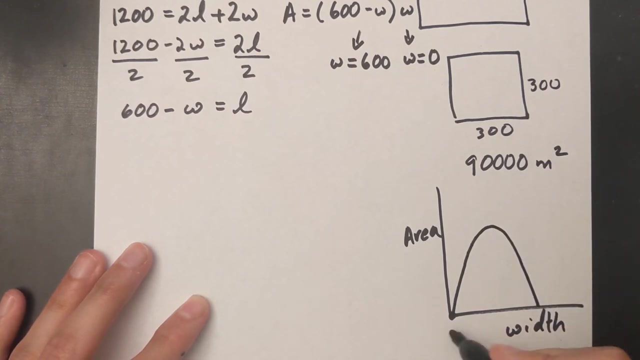 this one it's going to be w equals 600 and for this one it's w equals zero. So let's think about this on a graph. I have a graph here for my area, and over here is my width, and this equation looks like this: It's a quadratic equation. This is zero and this is 600.. 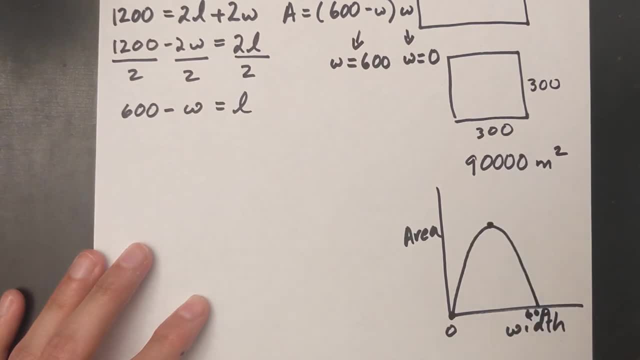 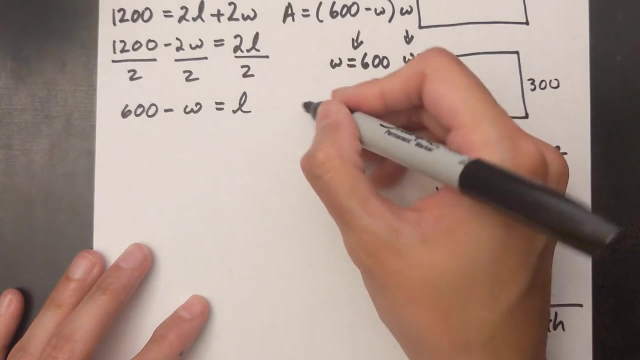 I need to find my maximum area, So that's the y value of this equation. So basically, I just have to find my vertex. The x value of my vertex is just the midpoint here, So my x value, or my w, is 600. 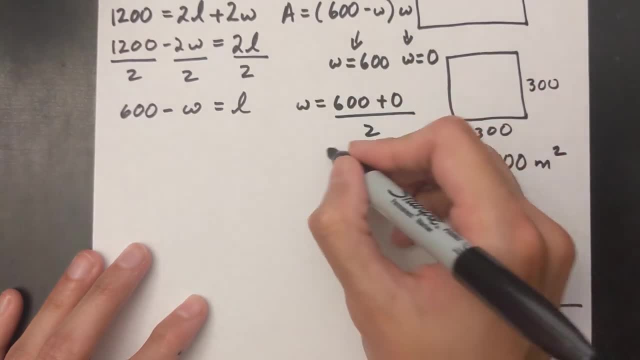 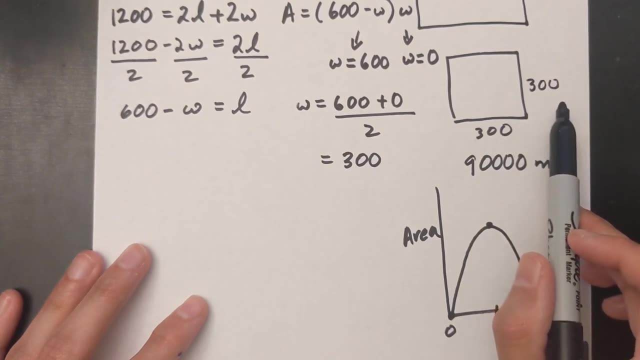 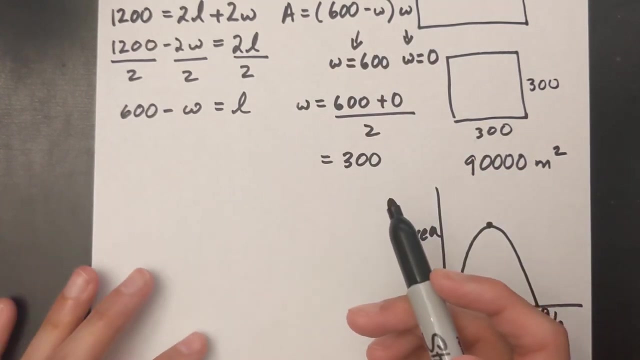 Plus zero, my two x intercepts divided by two, which is 300, and, as you can see, it's the same as what I showed in the square. Now I just have to sub this into my area equation. I can also find my length if I want using this one. There's two ways to do it. It doesn't really matter, I'll find my length. 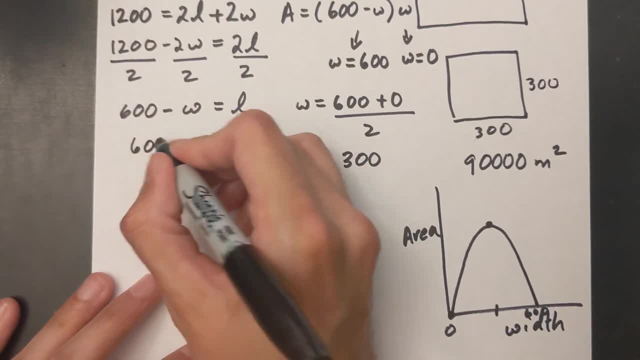 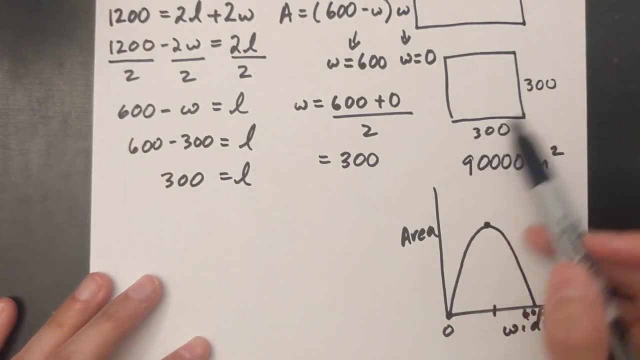 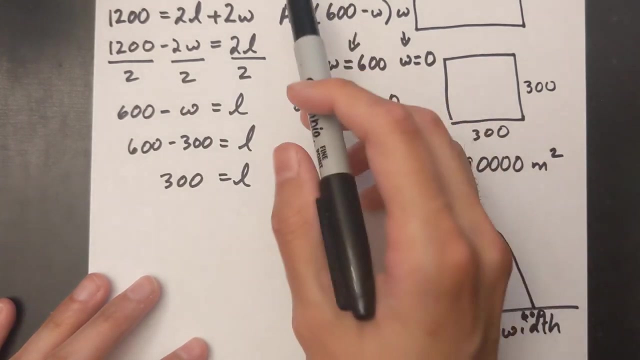 here first. So 600 minus 300 is my length. So 300 meters is my length. So, as you can see, that's what I've shown here. with this square, Your width and your length- I've proved algebraically- are exactly the same. All I have to do is sub it in my area: equation. 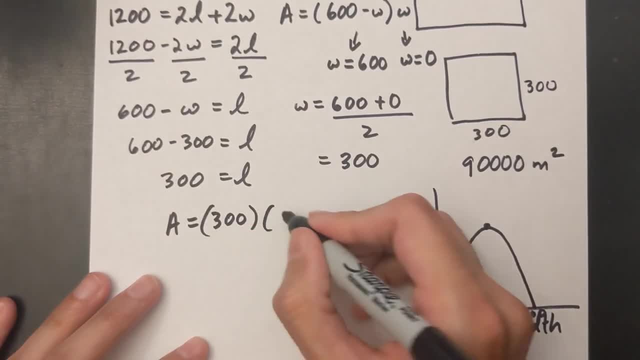 So area is length times width, which is the exact same solution there as 90 000 meters square.